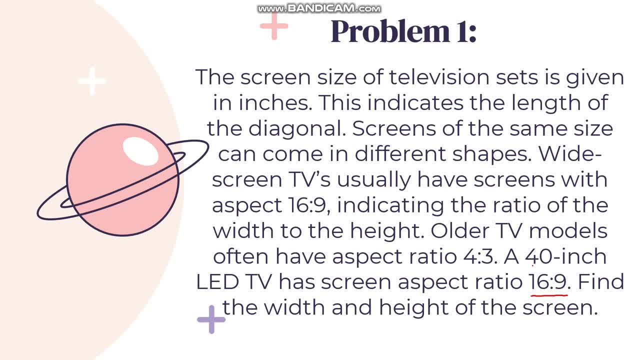 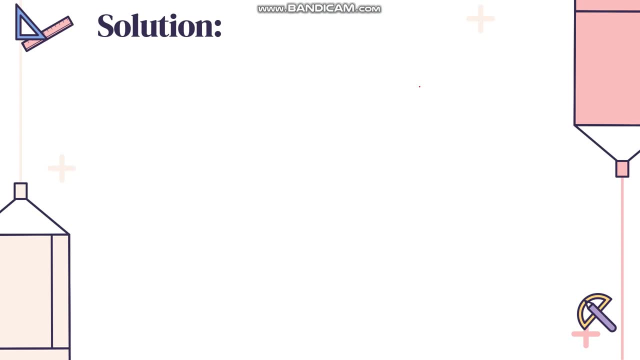 Now, given that a 40-inch TV has an aspect screen ratio of 16 by 9, now we have to find what is the width and what is the height of the screen In order for us to solve this problem. we have to to illustrate, just like how we do it with other word problems. So take note, We are considering a 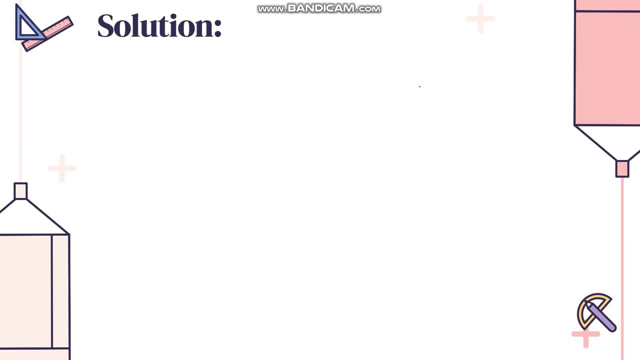 television, wherein its screen aspect ratio is16 by 9.. So let's say we have this rectangle that represents the television, And from the problem we also know that the size of the screen is 40 inches. And whenever we measure the size of the screen we are actually looking at the diagonal. so again, it's 40. 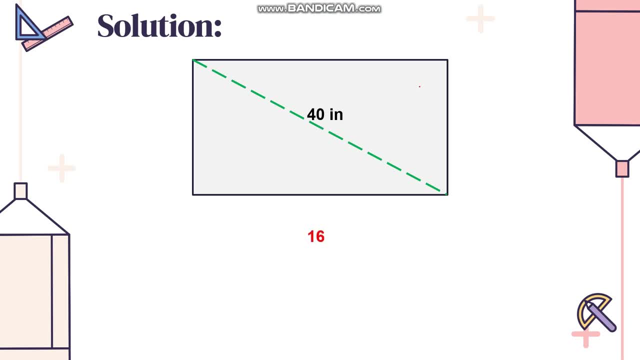 inches. you can take note the screen aspect ratio of the television that we are considering in this word problem is 16 by 9.. now the problem is we have to identify what is the width and the height of the given television. so we have to set variables for the width and also for the height. 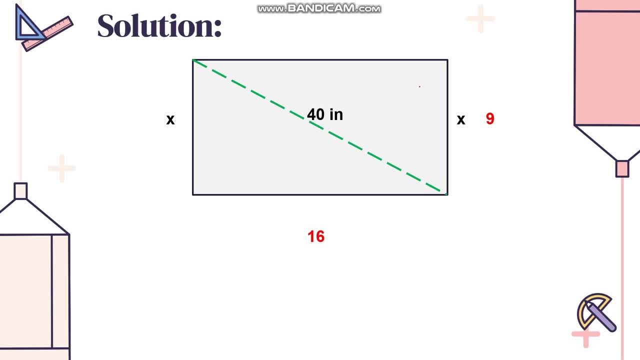 we can set x as the height of the television, so that means both sides of this rectangle should be x, because of course they should be stick one. and we can set the width as y, so the bottom and also the top part here is also y. so this is now the illustration of our word problem. 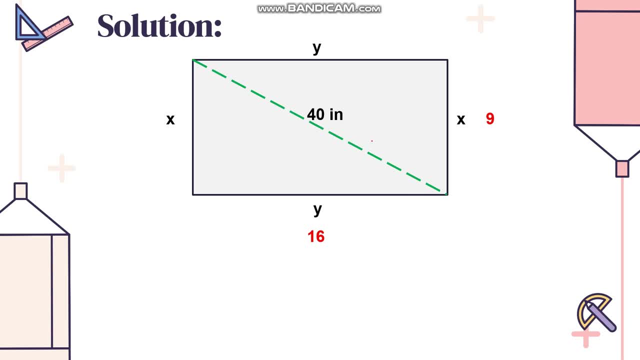 now, from here we have to construct equations, non-linear equations, so that we can solve what is the value of x and what is the value of y, because x and y represents the height and also the width of the given television. so what we know first is that this television follows a ratio of 16 by 9, so ratio can also be. 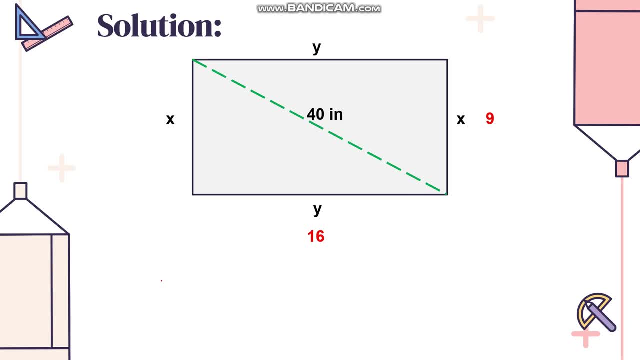 written in fraction form. you are thinking about ratio of 16 by 9. that means it's 16 over 9, and we know 16 is for the width and then 9 is for the height of the television. so with that we can actually write our first. 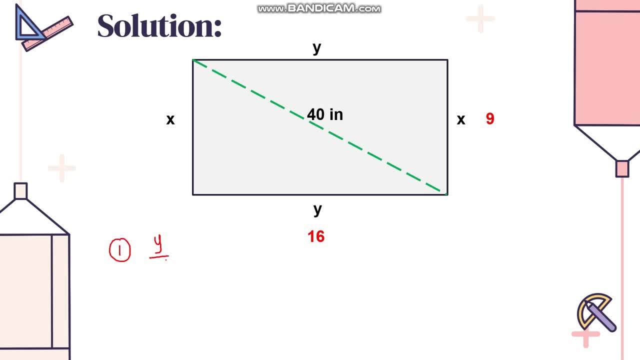 equation as y over x. so you're getting the ratio of the width by the height and that is 16 by 9 or 16 over 9. so again, our first equation came from the given that this television follows a ratio of 16 by 9. and again, when we're talking about the screen aspect ratio we are looking at 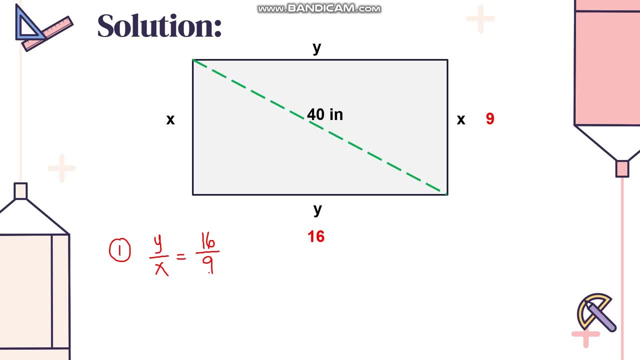 the width and the height of the television. so that's why it's y over x, equals 16 over 9. now we have to create another equation using the figure that we created. so what we can do is we can look at the width and the height of the television and we can look at the width and the 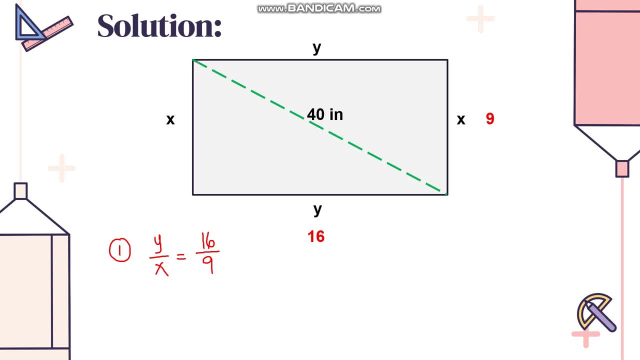 height of the television and we can look at the rectangle here and, as you can see, after we put the diagonal, there are now two right triangles form. so this one is a right triangle. this one is also a right triangle. so in writing our equation, we need to have the x and y variables. 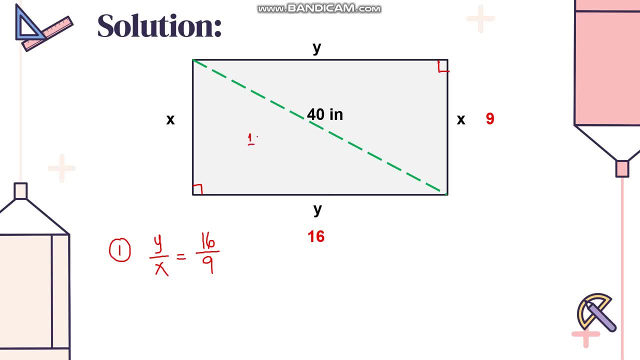 so we can consider this first triangle here, wherein x is one of the legs, y is also the legs and the diagonal here represents the hypotenuse of the given triangle. so we can use the Pythagorean theorem to create the second equation. so that will be: x squared plus y squared equals 40 squared. now, x squared plus y squared. 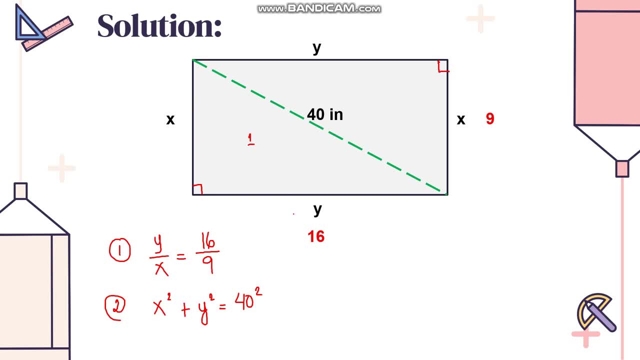 again, this follows the Pythagorean theorem: a squared plus b squared equals c squared. so you're adding the squares of the leg and it should be equal with the square of the hypotenuse, which is equal with the centuş cricket. so this type of equation in receives unnecessary. 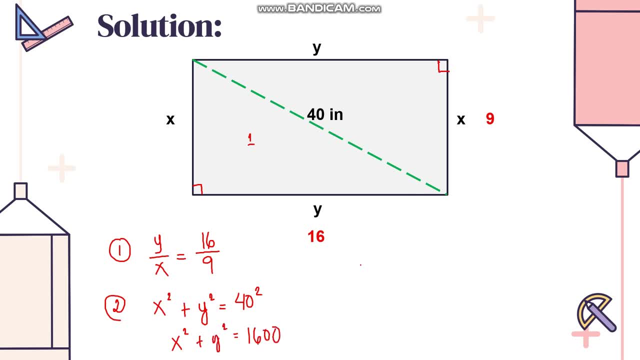 number, the deverb of the line can be separated. barbarian algebra: we're from point b over x or one over y. so we can figure out how to do that. now, if we want this, сделать a vy. now this equation number two, we can also write this: ask x squared, thus Y squared equals 1600. 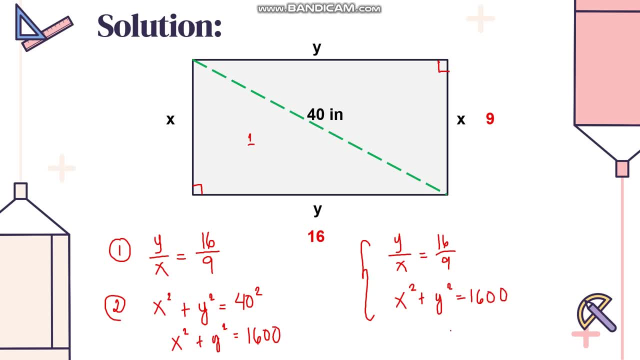 so we can write the system as: Y over x equals sixteen over nine, and the other equation is: x squared plus y squared equals 1600. so this is now our system of nonlinear equations. so we will be Now this equation number two. we can also write this as: x squared plus y squared equals 1600. then we put a list of numbers. 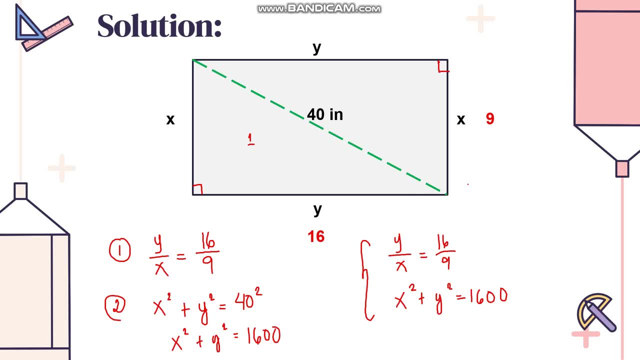 values of x and y. again remember: x is or, x represents the height of the television and y represents the width of the television. so let's just write here the equation we have: y over x equals 16 over 9. and then the other one is: x squared plus y squared equals 1600. 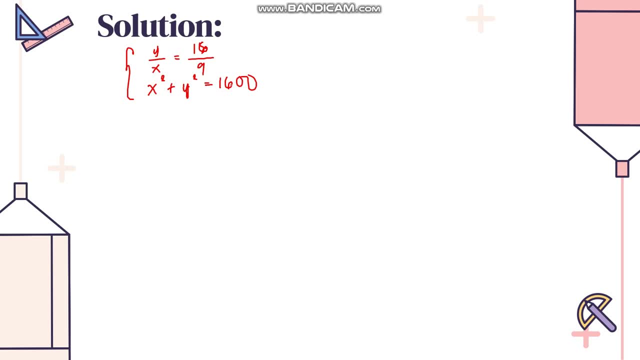 now we have to identify what method are we going to use- substitution or elimination? so in this case it's better if we will use substitution, because, if you will look closely at the variables given, on the second equation the variables are squared, whereas on the first one they are not. so it will 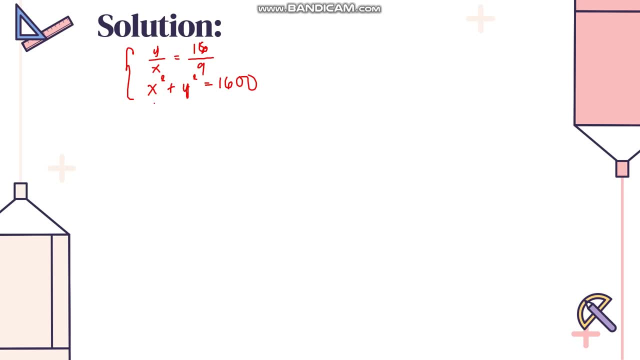 be a bit difficult for us if we will use elimination, since in the first place the variables are not the same, so we can just write here the equation we have: x squared plus y squared. use equation number one and let's try to use substitution. so using equation number one, which 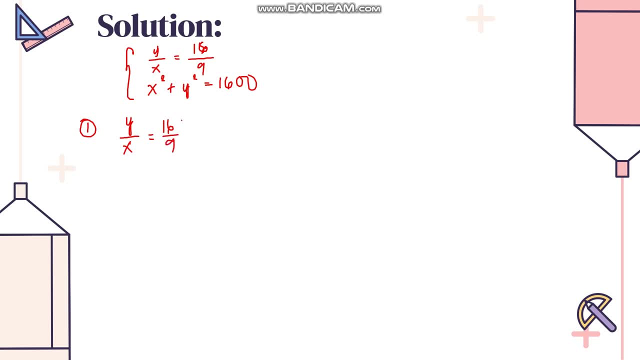 is y over x equals 16 over 9. we have to manipulate this so that we can isolate one of the variables. so to do that, we can just multiply both sides by x. this will be cancelled. we have y equals 16 over 9 x, and then we will use this value and substitute it to equation number two, so using equation number. 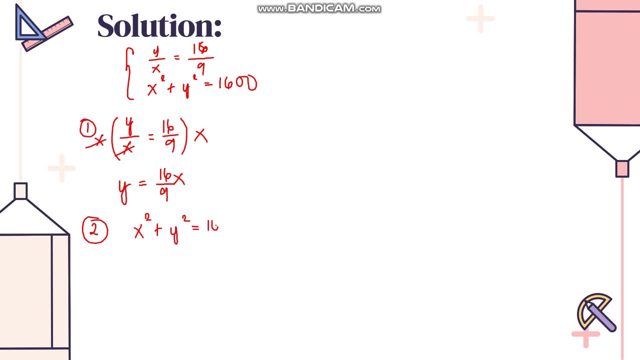 two x squared plus y squared equals 1600. let's substitute the value of y, so we have x squared plus 16 over 9 x, and then squared equals 1600. and then simplify this. we have x squared equals, or x squared plus 256 x squared. 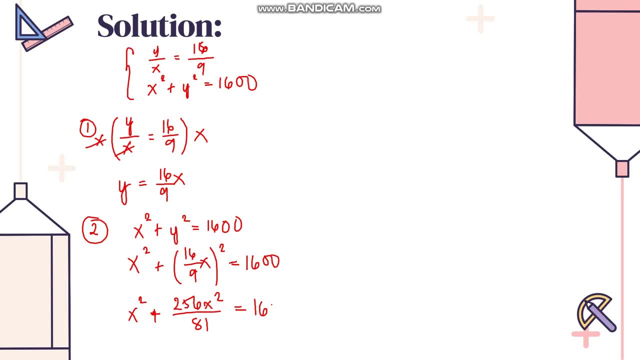 all over 81 equals 1600. now to remove the denominator or to remove 81, let's multiply both sides of the equation by 81. multiplying both sides by 81, we will get 81 x squared plus 256 x squared equals 1 600 times 81 is 129 600. 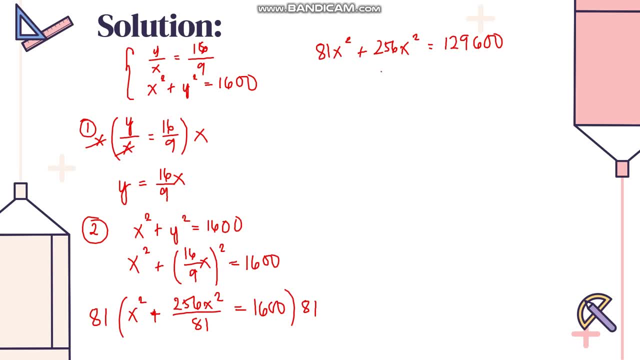 from here we can add a 181 and 256, that is 337. x squared equals 129, 600. and then next is: we will just divide both sides by 337, 337, so we have x squared equals. then this one, let's just write this as 129 600. 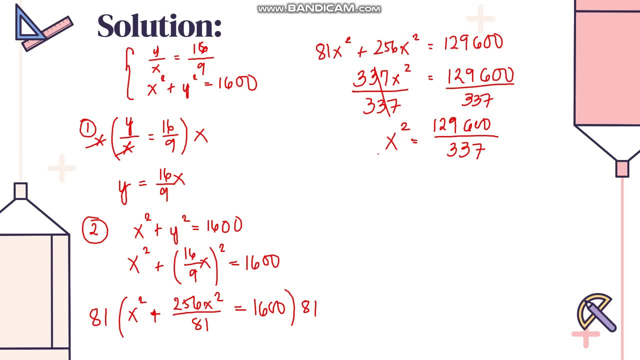 over 337. and then next is we have to get the square root of both sides, so this will be x equals. now let's just write it as square root of 129 600 all over 337, or if we will simplify this, we will get 19.61 inches. so this is now the value of x. 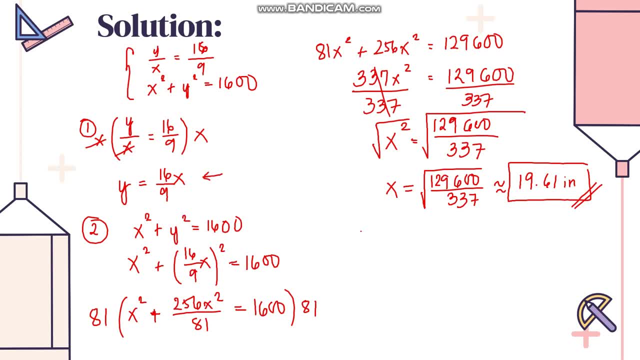 now to solve for the value of y. we will use this equation right here. so y equals 16 over 9 x. now to solve for the value of y. we will be using this value right here, because 19.61 is already the estimated value. so, to be exact, let's. 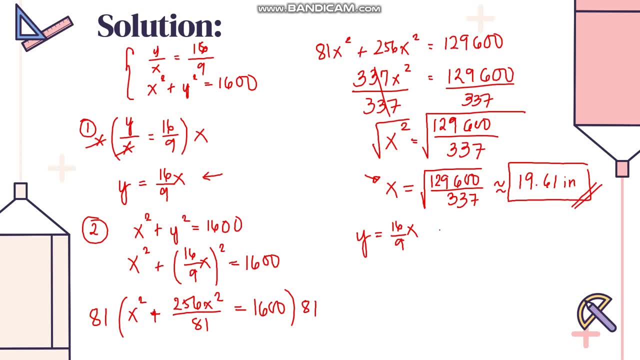 just use this one: the square root of 129 600 all over 337. y equals 16 over 9 times square root of 129 600 all over 337, and let's solve this using our calculator, so we will have 34.86 inches. 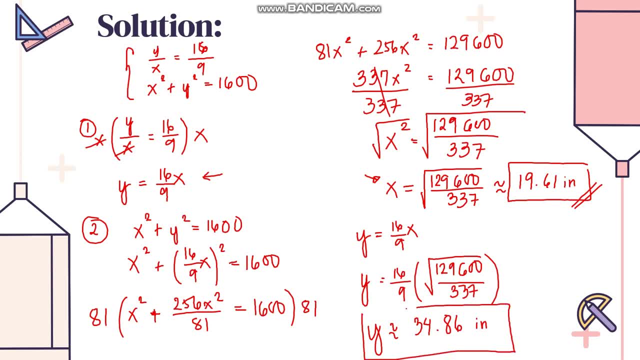 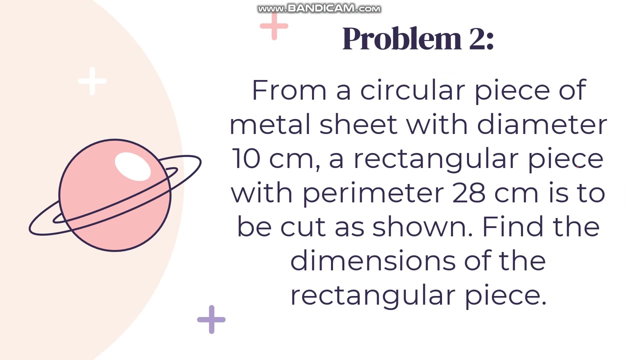 as our final answer. so this is now the value of y. so therefore we can say that the width of tv is 34.86 inches and length is 19.61 inches, and then this will be our final answer. let's have this second problem from a circular piece of metal sheet with diameter 10 centimeter. 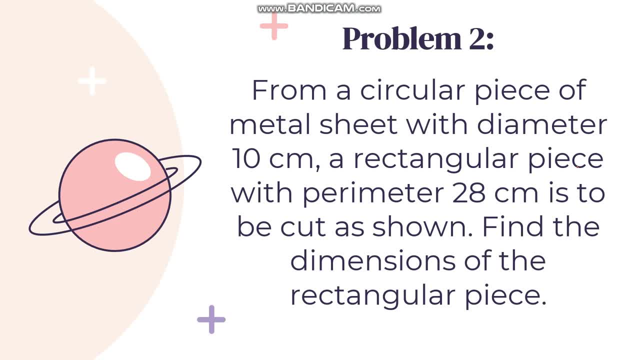 a rectangular piece with perimeter 28 centimeter is to be cut as shown. find the dimensions of the rectangular piece with diameter 28 centimeter is to be cut as shown. find the dimensions of the rectangular piece. if you will imagine this word problem. so there is a circle and inside the circle 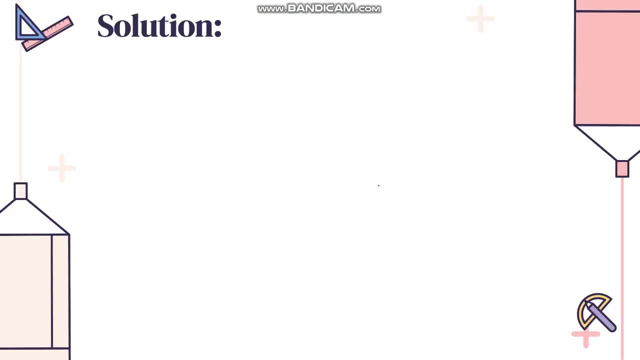 is a rectangle. so to illustrate the word problem again, we have circle whose diameter is 10 centimeter and inside the circle is a rectangle whose perimeter is 28 centimeter. so we know that the perimeter of rectangle is 28 centimeter. so now we have to identify what will be the dimensions of the rectangular piece. 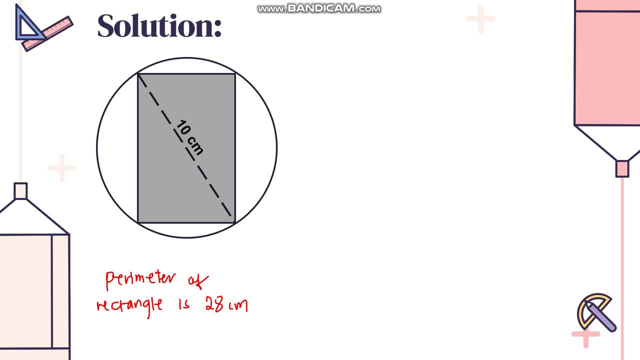 so that means we are looking for the length and the width of this rectangular piece right here, so we can assign values of, or we can assign variables to, the length and the width. so we can assign this side as x, so this one is also x, and then the other side here is y, so this one is also y. so again we are. 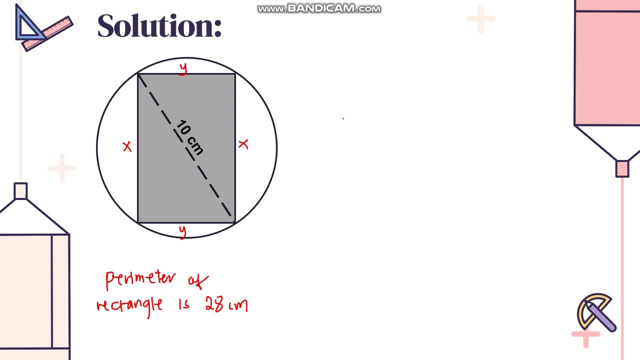 solving for the values of x and y. so let's now write the equation that represents or that we can use in order to solve this given word problem. first is, let's use this um concept that we know, wherein the perimeter of the given rectangle is 28 centimeter. now to recall also: 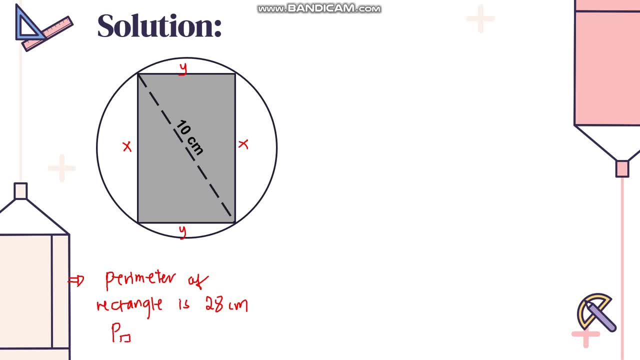 to get the perimeter of a rectangle we have to add 2l and 2w. that means you multiply the length twice, then you add also the product of the width times 2. so this is the formula. so we can use this in order for us to write an equation in this given word problem. we are going to write an equation. 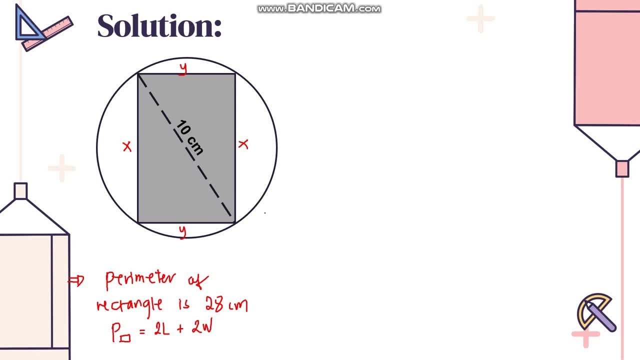 in order to write an equation in this given word problem. uh, we can see that the length is x and then the width is y. so we can write here: 2x plus 2y equals 28.. now remember x. we refer it as the length. 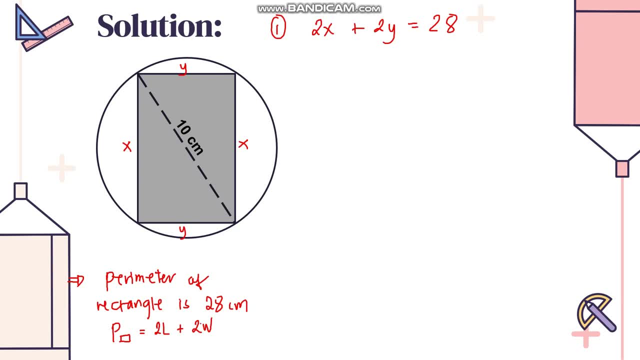 and the y, that is for the width of the given rectangle. so we have 2x plus 2y equals 28.. you can the two. it can be 2y plus 2x equals 28, so it doesn't matter. so this equation right here: 2x. 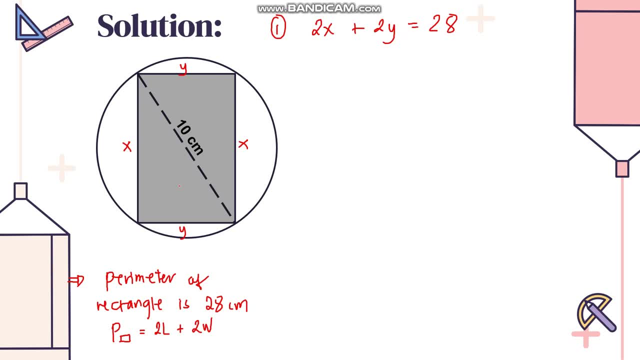 plus 2y equals 28, came from the, the perimeter of the rectangle. for our equation number two, like what we did with the problem number one, we use a right triangle. so, as you can see here, after we put the diameter of the given circle, there are now two triangles formed, so this one is a right triangle. 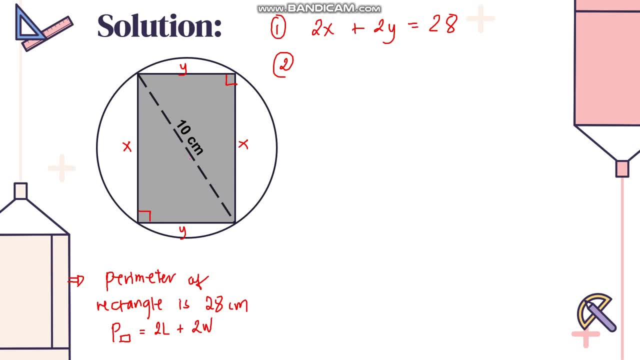 also, the other one is a right triangle, so we can use again the Pythagorean theorem. so these are the legs, and then this one is the hypotenuse. so you can write here: x squared plus y squared equals 10 squared, or this one is x squared plus y squared. 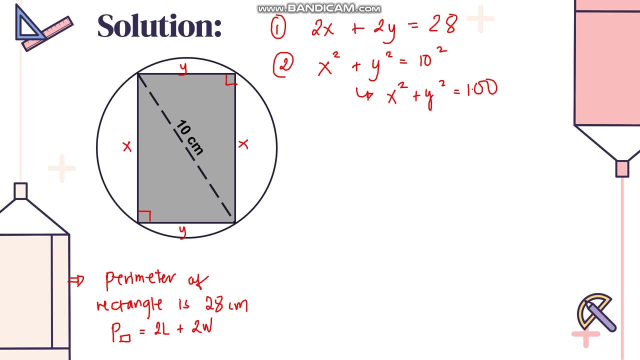 equals 100. so the equations, now that we have 2x plus 2y equals 28 x squared plus y squared equals 100. now, to solve this again, you can use uh, elimination or substitution. it's up to you what you will use, but for this case, since, if you will notice, the 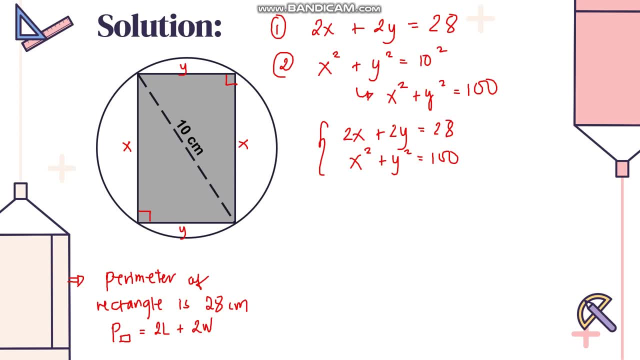 variables. in the first equation their exponent is just one. for equation number two their exponent is two. so that means they don't have similar variables. so it is better if we will use substitution. so we will be using substitution here and we will start with equation number one. 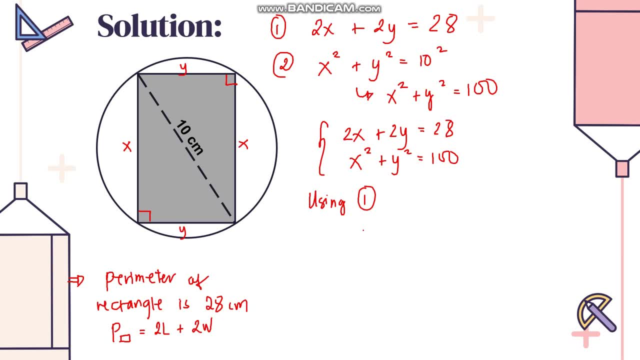 so let's use equation number one to have a value or a temporary value of x or y. so equation number one is: 2x plus 2y equals 28. so, as you can see, all of them is divisible by two. so we can still simplify. so 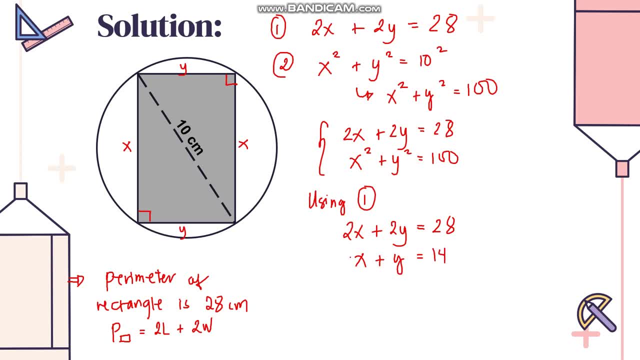 we have x plus y equals 14. it's either now here you move x on the other side or y on the other side, so it will be okay. so let's just move y on the other side, so that we can have x equals 14 minus y. so this is now the temporary value of x. 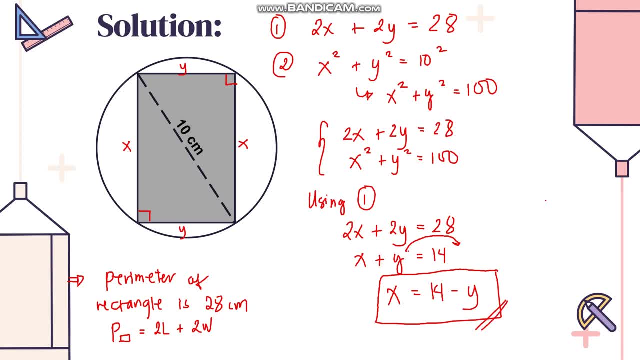 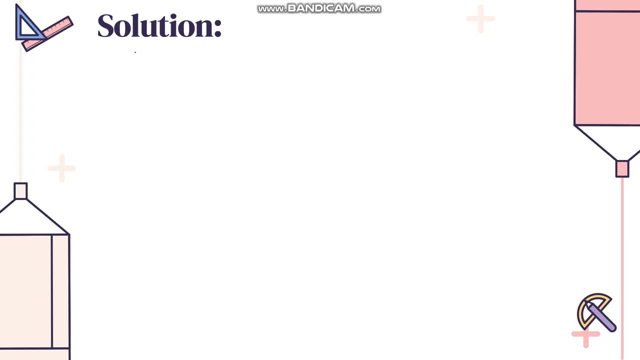 and then we will use this and substitute this to equation number two to identify the first variable, which is y. so to continue using equation number two. so let's now do substitution. equation number two is x squared plus y squared equals 100, and we have to substitute the value. 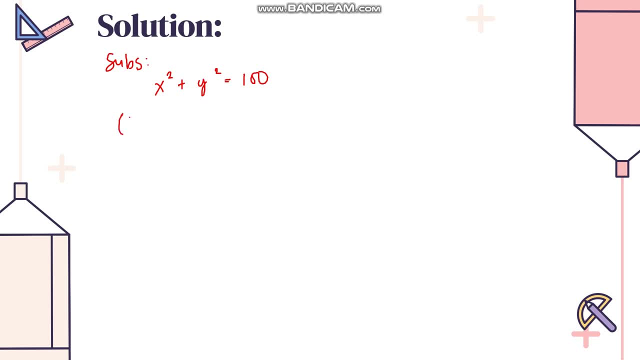 of x, which is 14 minus y. so here we have 14 minus y, and then squared plus y squared equals 100, and then you simplify this square of binomial, or you can do foil method: 14 squared is 196, and then 14 times negative, y times 2, that's negative 28, y plus y squared, and then 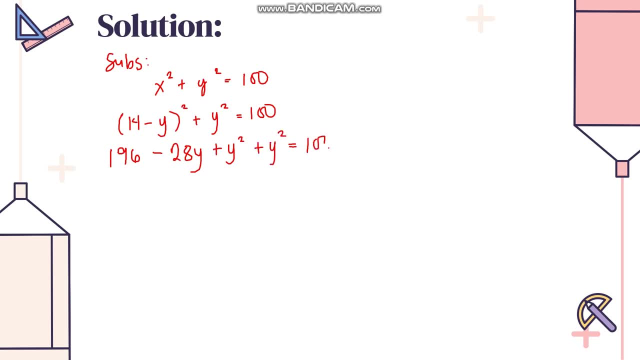 plus y squared again equals 100. simplify this: y squared and y squared, so that is 2y squared. so just copy 196 and negative 28 y and then we have here: plus 2y squared equals 100. we can rearrange the terms here, so we have 2y squared minus 28 y. 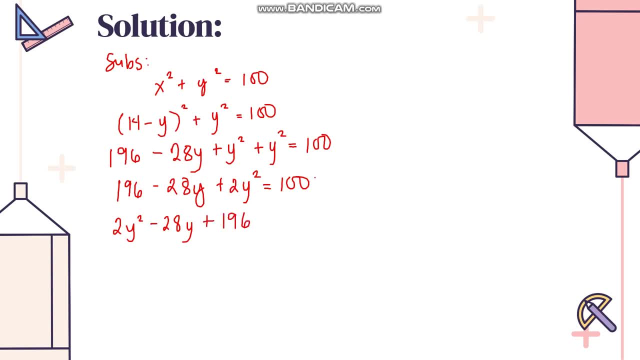 plus 196, then 100. we can move here on the other side. so we have minus 100, then equal to zero. after that we can simplify this two right here. so 2y squared minus 28, y plus 96 equals zero. now look at the terms of the given equation. so, as you can see here, all of them are: 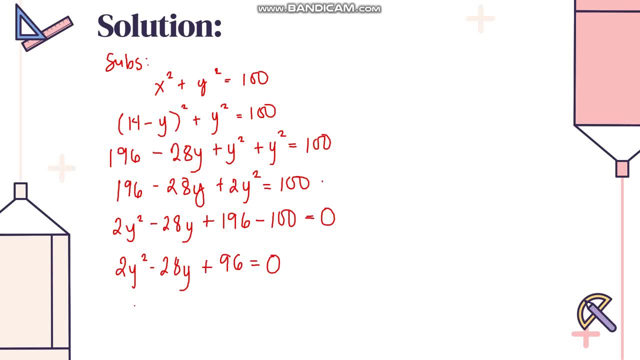 still divisible by two, so simplify them. so we have y squared minus 14, y plus 48 equal zero. now we now have a quadratic equation here, and in order to solve this we can use factoring. let's write here again: y squared minus 14, y plus 49 equals zero. now find factors of 48, that when you add the answer is negative 14. so we have negative 8 and negative 6, so the factors here will fit there. so we'll have –� 18 –6. so the factors here will fit that when it's plusские nosaic n2 –6, it'll be minusfull at 116 because we have minus 8 here. 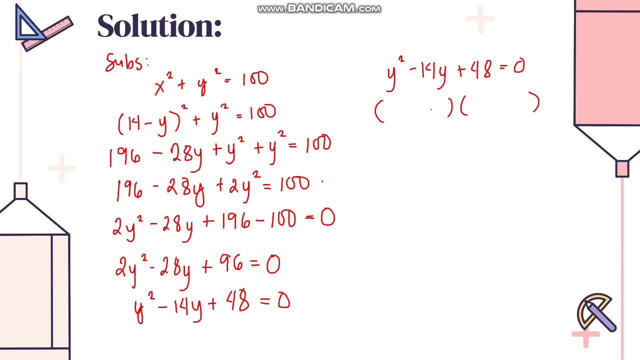 is negative 14, so we have negative 8 and negative 6. so the factors here will be y minus 8 and y minus 6 equals 0. then after that we can now equate each factor to 0, so we can get the values of y. 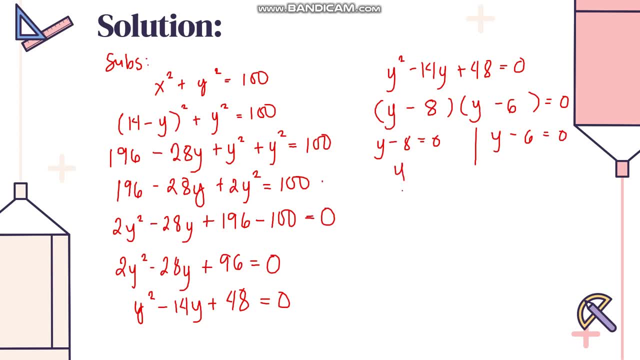 so this will be equal to y equals 8 and the other one is y equals 6. then after that we can solve now for the value of x. so, using the equation that we have x equals 14 minus y, let's solve for x. so, if y is 8, so we have x equals 14 minus 8. 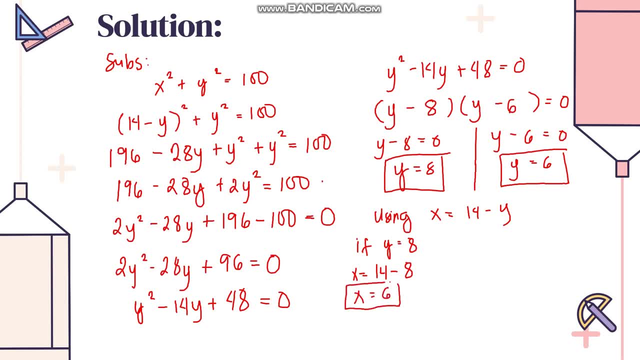 which is 0, so we can get the value of x, so we can get the value of x, so we can get the value of x is equal to 6. and then, if y is equal to 6, so we have x equals 14 minus 6, or x equals 8. 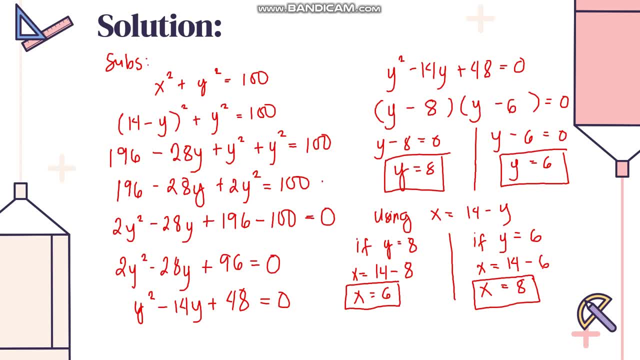 so now, as you notice, first pair here is y is 8 and then x is 6, the other one, y, is 6 and then the other one is 8. so it doesn't matter what we will do is we'll just consider one, since we're. 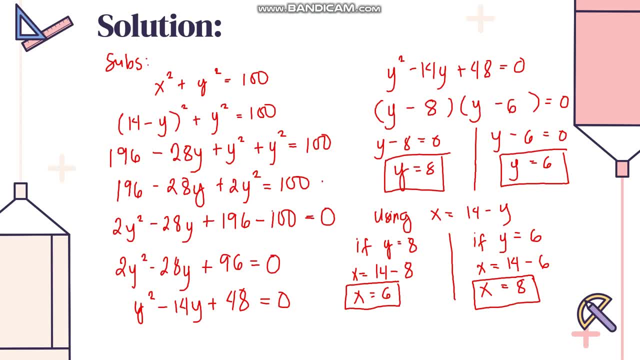 just asked by the dimensions of the rectangle. so for our final answer we can write: the dimension of the rectangle of the rectangle is 8 inches by 6 inches. so that will be our final answer. so we know that the dimensions of the rectangle is 8 inches by 6 inches.